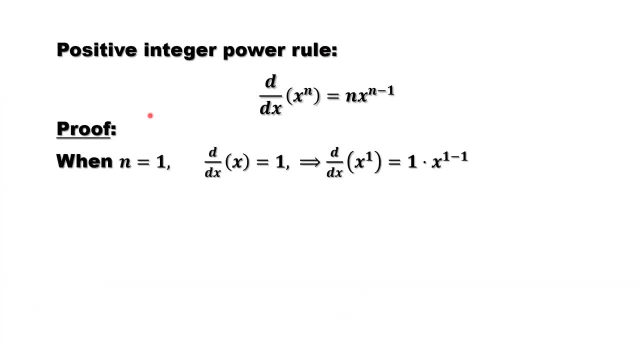 The first step. we need proof. this result is true at the starting point. What is the starting point Here? we are assuming n is an integer positive. So which one is the smallest positive integer? n equals one. So we need to check if n equals one. 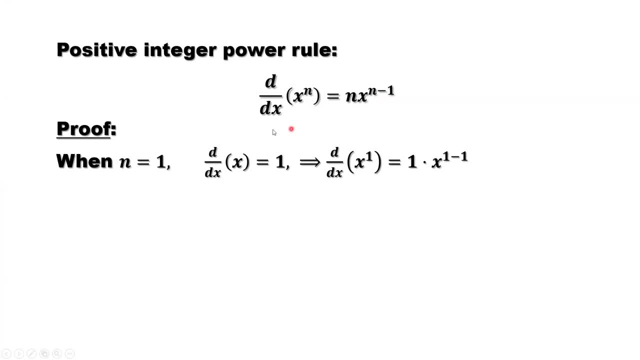 this result, if it is true, n equals one. left-hand side is derivative of x to the power one equals one time. x to the power. one to the power one. The power is zero. x to the power zero is one, So the right-hand side should be equal to one. 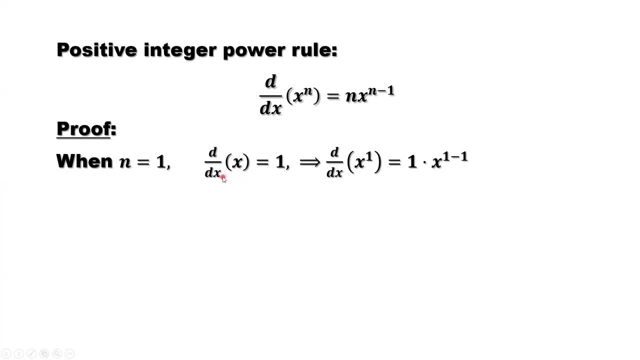 From the definition of derivative we know that The derivative of x equals one. Rewrite this in this way: Derivative of x to the power one which is x. The derivative of x to the power one is one here times x to the power one minus one. 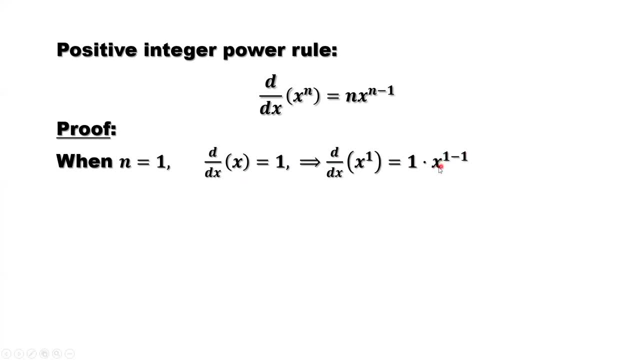 One minus one is zero. x to the power zero is one, So it is one, Same as right-hand side, left-hand side is the same. So here, when x equals one, this general result is true, Just to replace n by one. 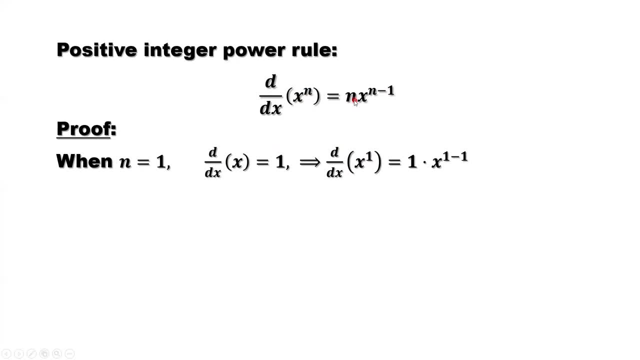 So x to the power one is here Right-hand side is one. One that's n times x to the power one. One that's n times n minus one, One minus one. This power rule when x equals one, it is true. 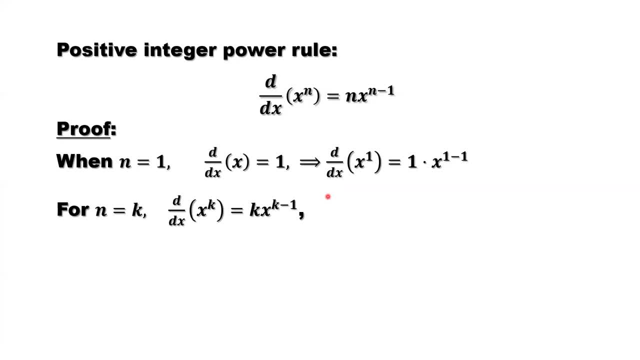 Now second step, based on the induction logic, if n equals k is true, can you derive: when n equals k plus one, This result is also true. So we are assuming n equals k it is true. That means the derivative of x to the power k. 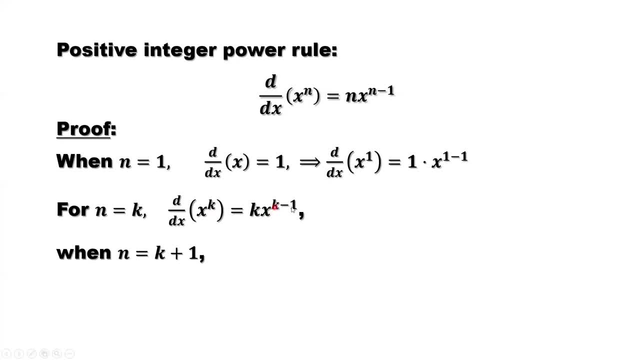 equals k times x to the power k minus one. We need to use this to derive this result: The derivative of x to the power k plus one. k plus one. we can rewrite as the product of x to the power k times x. 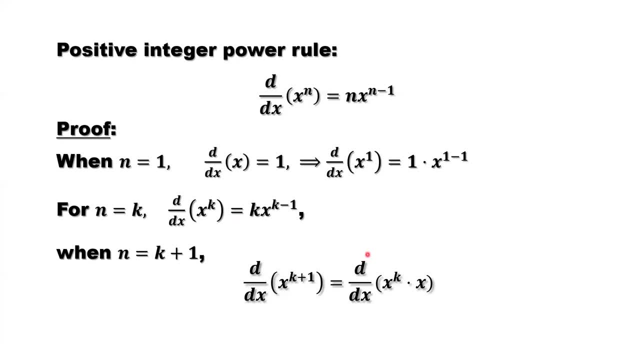 Use the product rule from calculus. So here the product rule is this: The derivative of the first term time, the second term plus the derivative of x to the power, k plus one. The derivative of first term time, the derivative of second term, The derivative of first term. 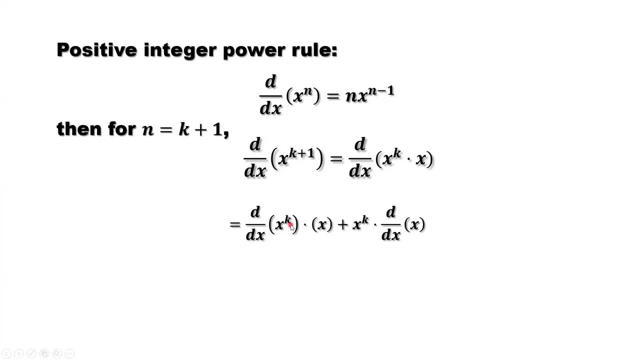 which is derivative of x to the power k. We can use the assumption when n equals k. we are assuming this case is true from the power rule. So that's k times x to the power, k minus one. Then times x, x is outside. 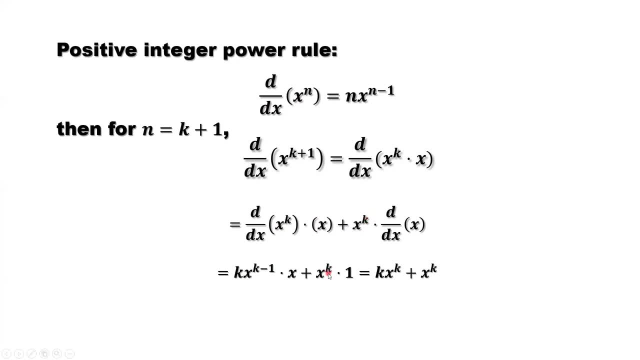 Plus x to the power k times the derivative of x, which is one Simplify. we have k: x to the power k plus x to the power k. So we only have x to the power k here. He has k, he has one. 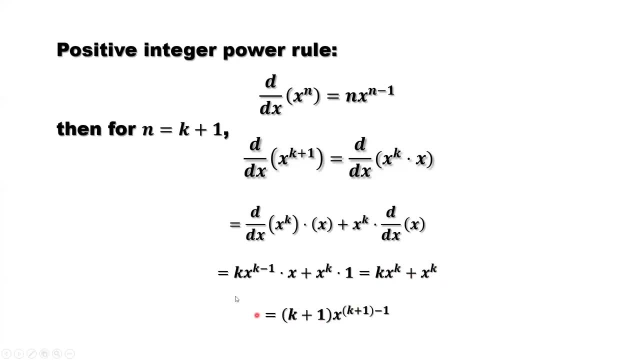 Put them together, it's k plus one. So k plus one x to the power k, x to the power k is equivalent to k plus one minus one. We need to rewrite this kind of format to compare with the original result. So original result is this: 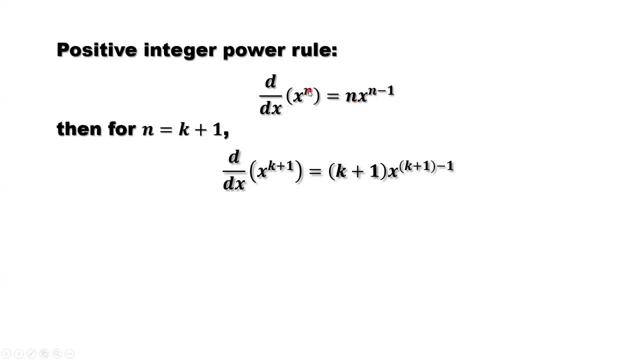 n. he has n minus one. So here, if he has k plus one, here should be k plus one minus one. So here, when n equals k plus one, this result is also true. You can see here if n equals k plus one.